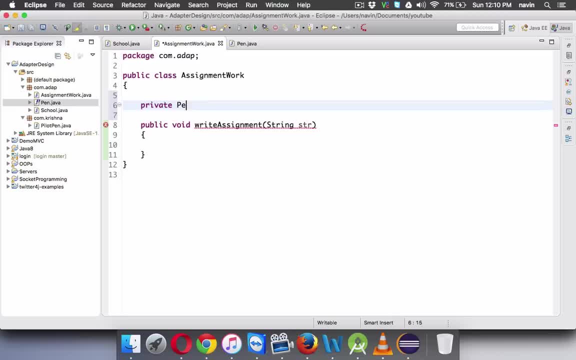 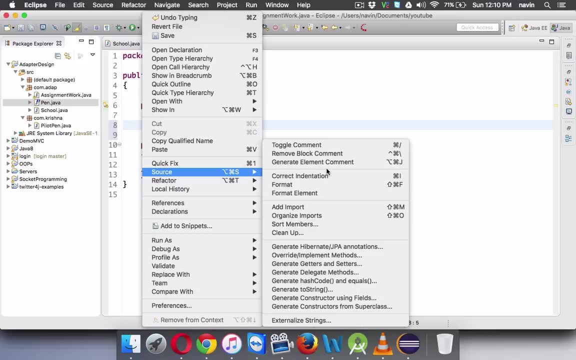 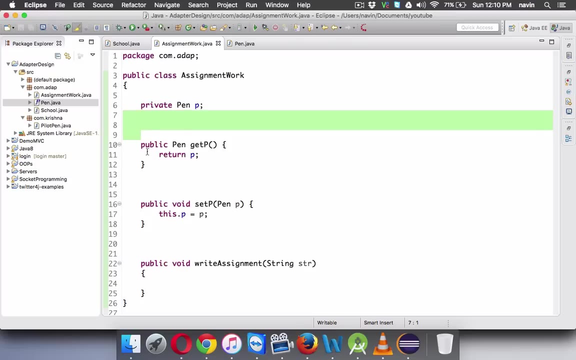 pen. no, private, yeah, pen p. we got private pen p. now, since it's in a variable, we require getter setters for this. we'll right click. we'll say source: give me a getter setter for p. okay, we got the getter setter for p. I hate these extra spaces given by eclipse. I don't know why. 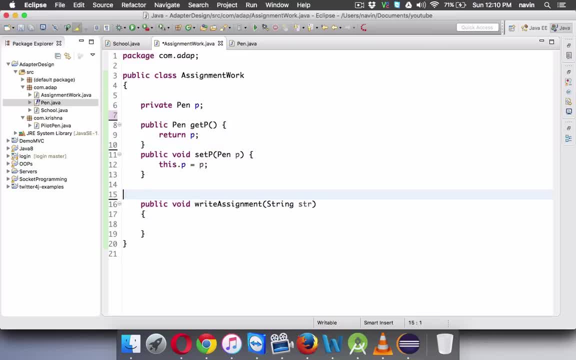 eclipse provides these spaces. okay, if you know this, just comment in the comment box below in the comment in the comment section. if you know how to solve this problem in eclipse, okay, so now. uh, so from this, what we need to create is we need to create object of assignment. 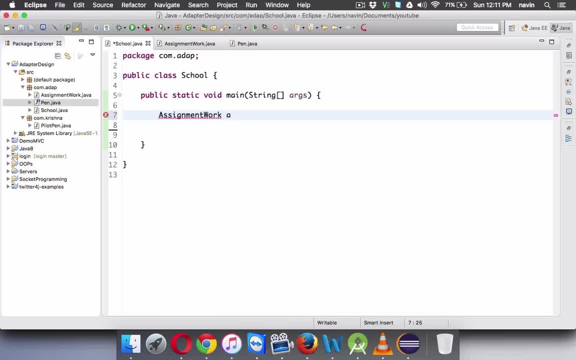 uh up assignment work and we'll name this as aw equal to new assignment work. okay, that's that. that's there, and then we can call aw dot what write assignment and we can pass i am tired to write an assignment, okay, so we need to print this. so if I run this code, 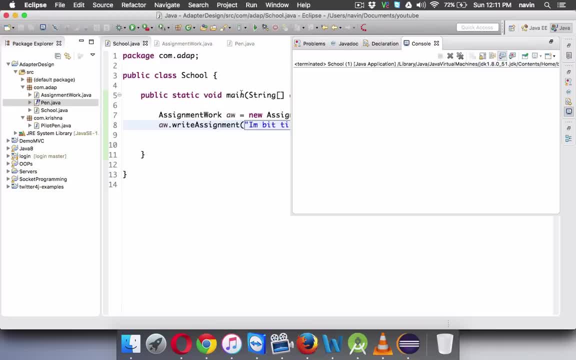 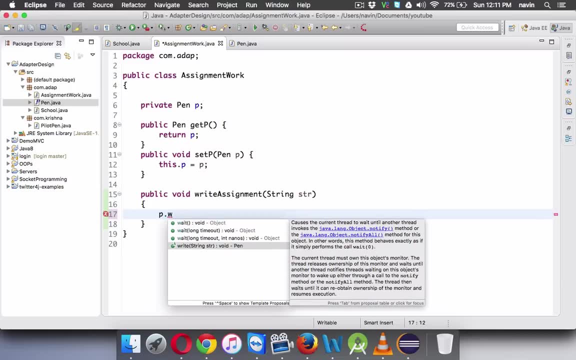 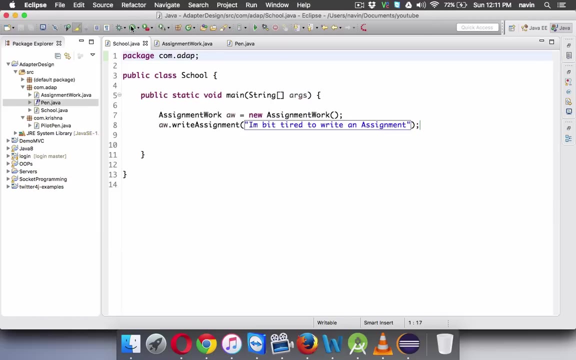 uh, we got an error here, which is: oh, we got nothing because, because, because we are not writing anything, we have to write, say p dot, p dot, right, right. we need to pass this string here. and if I go to school, because pen will write as a, as a normal user, we don't write right, pen writes. 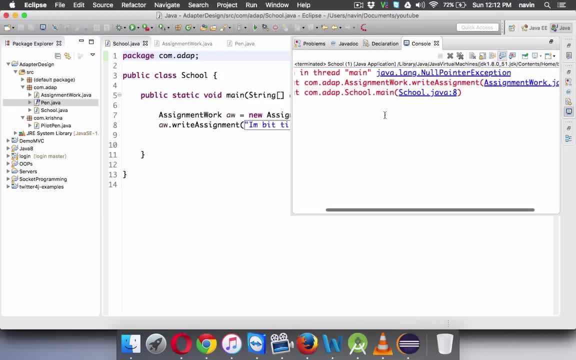 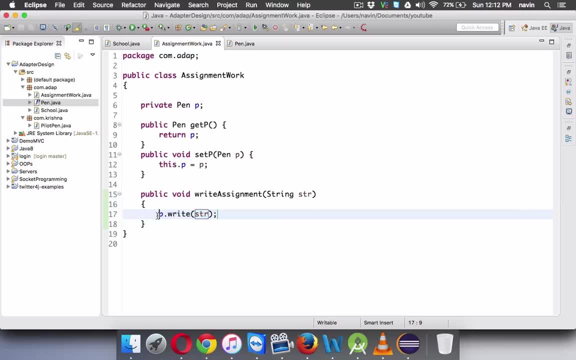 the data. so if I go to the this uh output, you can see there's another pointer exception. the problem is we are calling right assignments, which needs an object which is p, because using p, which is, we are saying p dot right, but we have not assigned the memory to p, right, so we 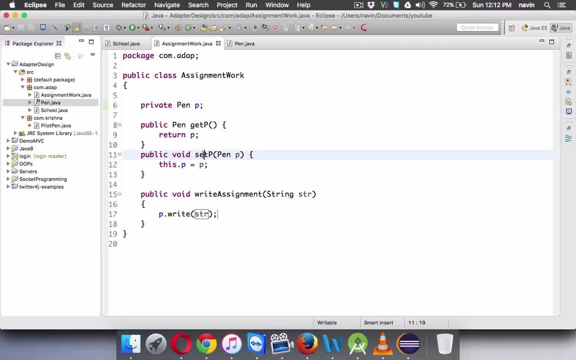 need to assign the memory. so to assign the memory, we have to call set p so we can say aw, dot, set p and we need to create object of pen. but hold on, I don't have the uh pen is the interface and I don't have the implementation. 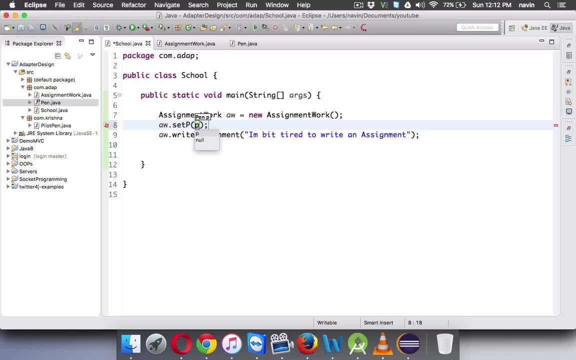 for pen. Maybe to create the implementation for pen, I have to create a method which is right. I want to. I have to set the properties- the size of your pen, the width of your nip and all those things- right, We need to set lots of things And I'm very tired to create. 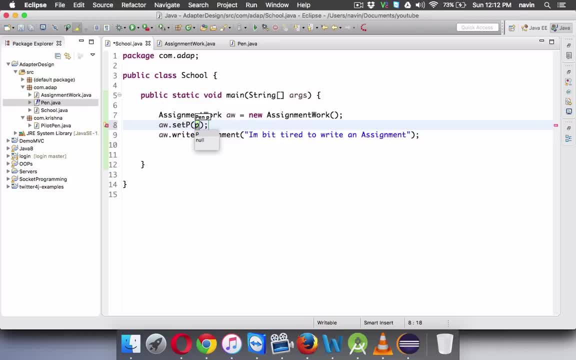 this object. So I call my, because anyway, when you go to college or school you never carry your pen right, You never carry your own pen. You ask your friends to give you that pen. So I called my friend and said: I want the object of pen interface. And he: 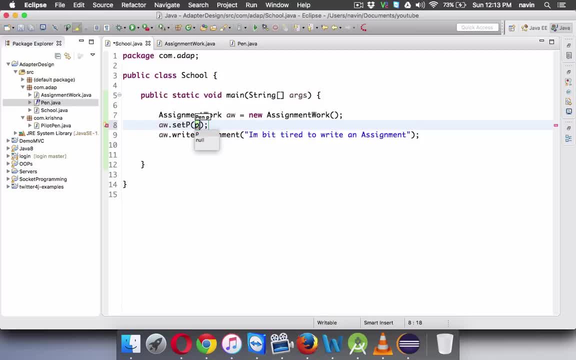 says: oh, I don't have the object of, I don't have the class which implements pen interface, and why should I create a pen interface for you? But I have a class. okay, I have a class which is pilot pen, which has nothing to do with the pen interface. So if you open pilot, 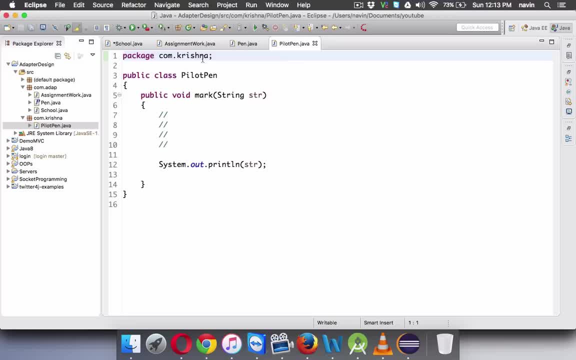 pen. it has nothing to do with the pen interface. You can see that my friend's name is Krishna. He has nothing to do with pen interface, Okay. So I said, it's okay, You can. you can just give me the object of. you can just give me. 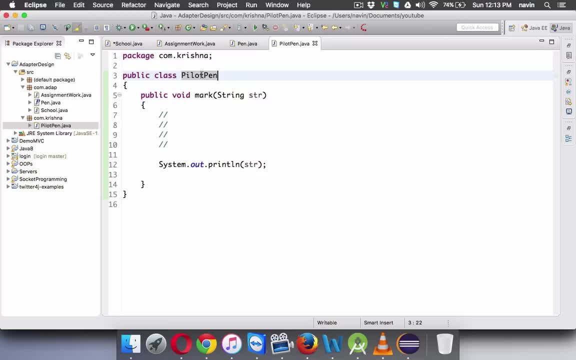 the class for pilot pen, And he's very smart. He's not giving me the source code. Okay, I thought he will give me the source code. I will change it. I will change the source code, But unfortunately he's not giving me the source code. What he gave: what he gave. 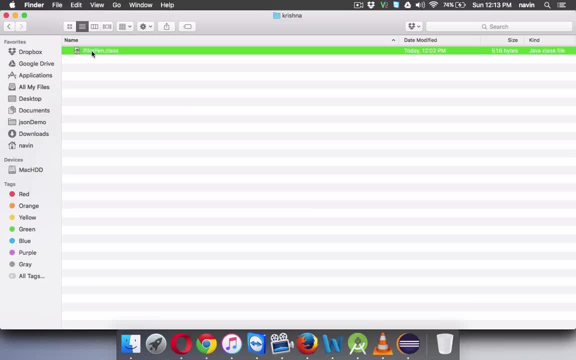 me is the class dot class file which is pilot pen dot class. That's weird, right. Maybe he's a friend or enemy, I don't know. He's giving me this thing which is pilot dot pen, pilot pen dot class, which I cannot change. So even if I create object of pilot, 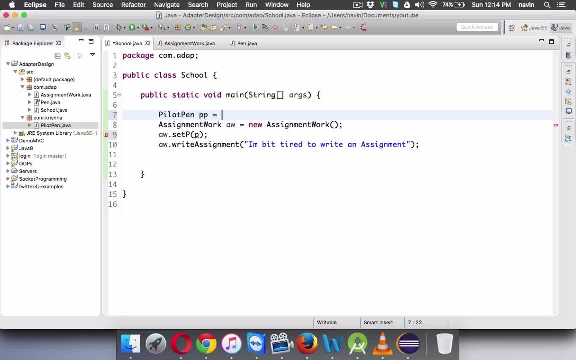 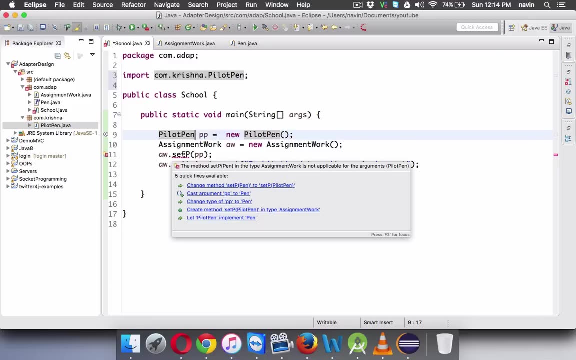 pen, pp equal to new pilot pen, which is pilot pen. And if I pass object pp here, okay, First need to import the package. Okay, Package is imported. Now you can see it gives an error Because we are passing object of pilot pen And here 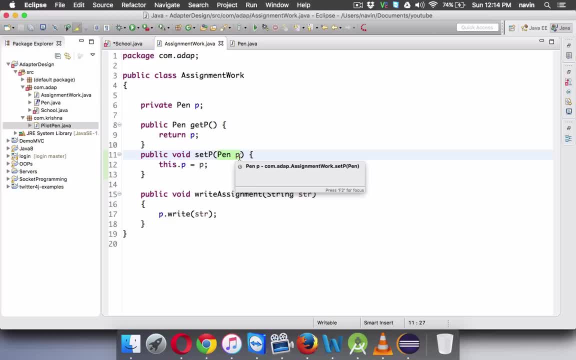 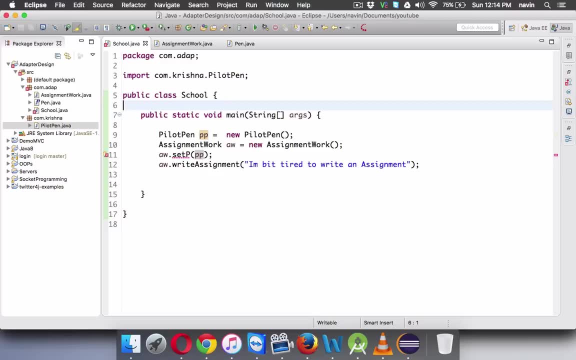 you're accepting pen. how will that work now, okay, so we cannot. we cannot do that right. we cannot pass object of pilot pen. so it this? the problem is same as, let's say, you have an iPhone and you want- your battery is bit low- you want to charge your iPhone and 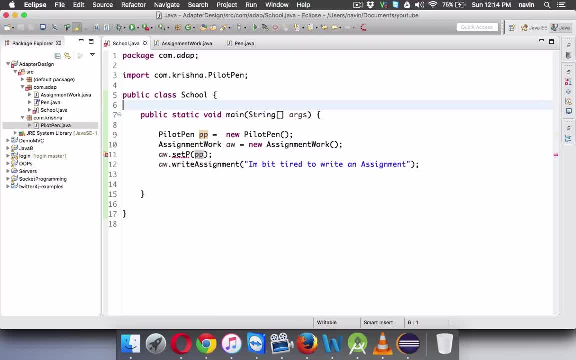 you don't have an iPhone charger. so you went to your friend house and then said: I want the charger. so he has. he is using a Samsung phone, so he got a Samsung charger. now you cannot connect a Samsung charger to iPhone, right? so we require an adapter so that adapter. what that adapter will do is you can connect. 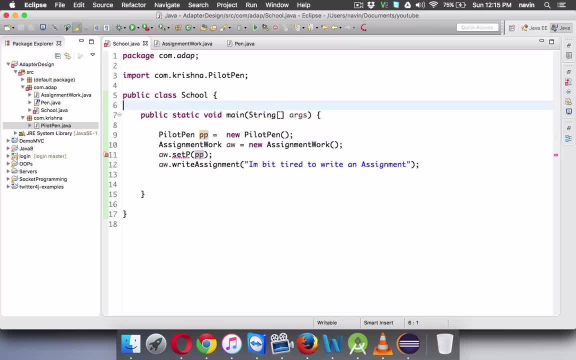 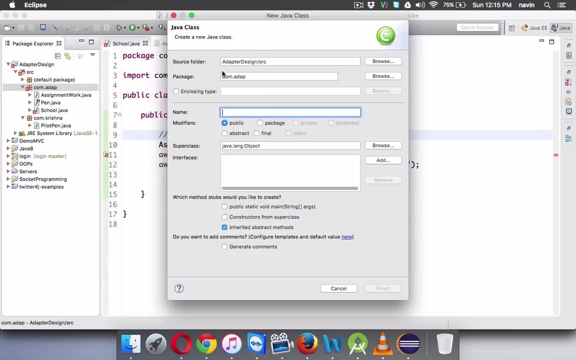 the Samsung charger to the adapter, and that adapter will be connected with your iPhone, so we require some something in between. we cannot pass object of pilot pen here, so that's not possible. but what we can do is we can create a class. we can create a class here which will, which will be called as the pen adapter, which 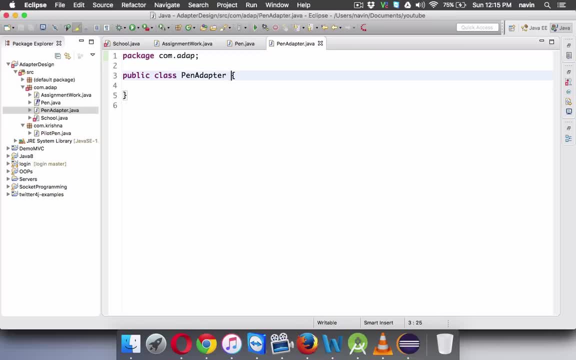 can take any type of pen, maybe a pilot pen or an ink pen, maybe a gel pen. so in this will be having also, this adapter will implement a pen interface, so this will implement pen interface. since we are implementing pen interface, we need to implement all the methods. okay, hold on, that's way to implement all. 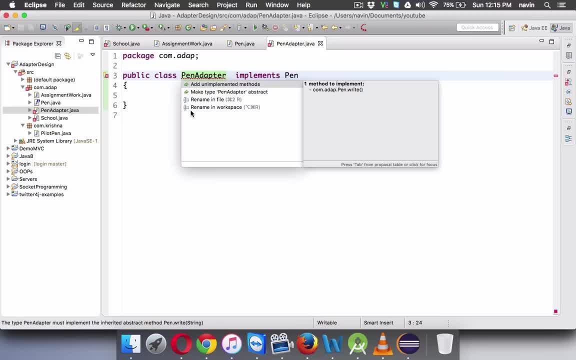 the methods. so we have to say implement, okay, implement all the methods. and well, now we can say, okay, hold on. but I, I don't want to define all the method, all these statements here. so my friend has given me the pilot pen of pilot pen class right, so I've got to, will do, I will say pilot pen. 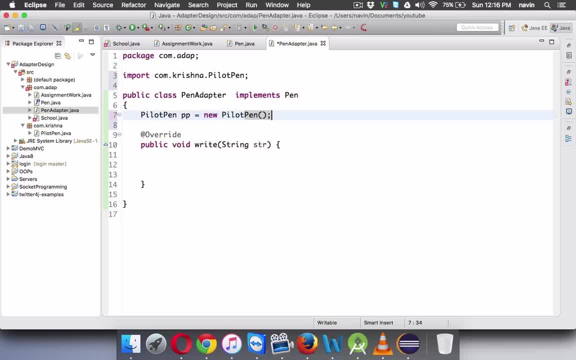 PP equal to new pilot pen. I will use his implementation using composition and I can say PP dot mark, since the depth, the method in this is mark. right, at least I have that. access to the to call mark sounds good, right, so we got PP dot mark and then from this, instead of passing the object of pilot pen, let me get an. 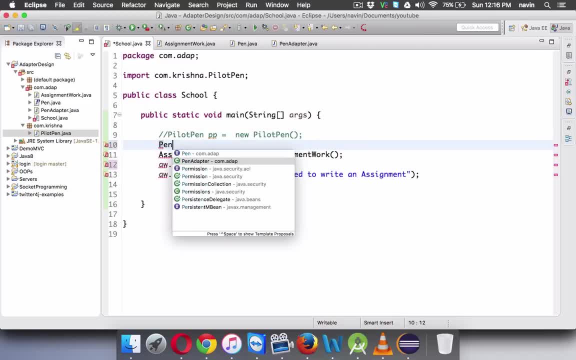 object of a pen adapter which implements pen. so we'll say we can even say pen P equal to new pen adapter, and then we can pass the object of p here, our object be here. okay, and now if I run this code we got, I am bit tired to write this. write an assignment. 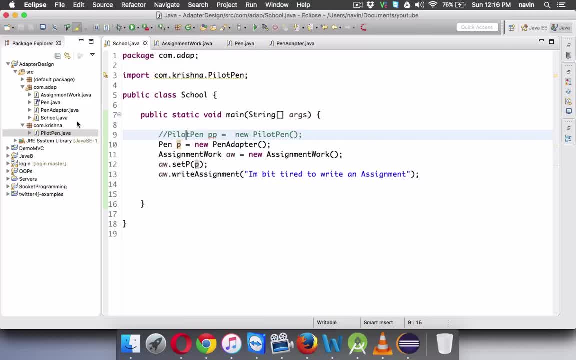 so that's the awesomeness about adapter. so my friend is giving me just a class file and I'm trying to connect the his class file or his implementation, which I required. so I have a pen interface and I want the implementation. I'm using his. 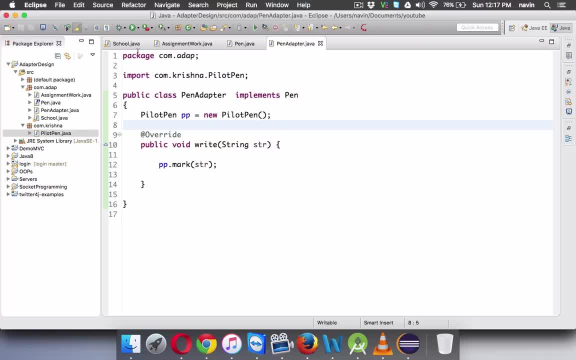 implementation with the help of adapter in between. yeah, so that's your adapter design pattern it's. initially it will be difficult to understand. i think you'll be watching this video two or three times to understand what exactly is going on. but just to make sure, watch this video and practice your own examples to master the design pattern. 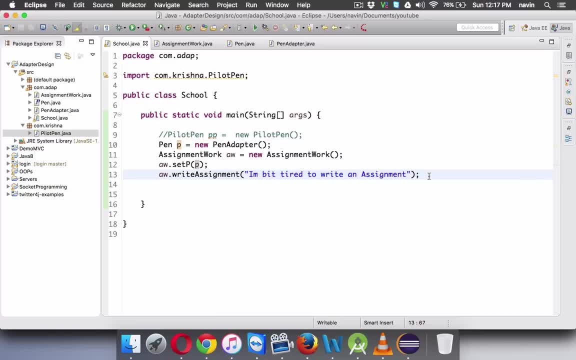 ok, so that's it from this video. make sure you subscribe the channel for other videos.